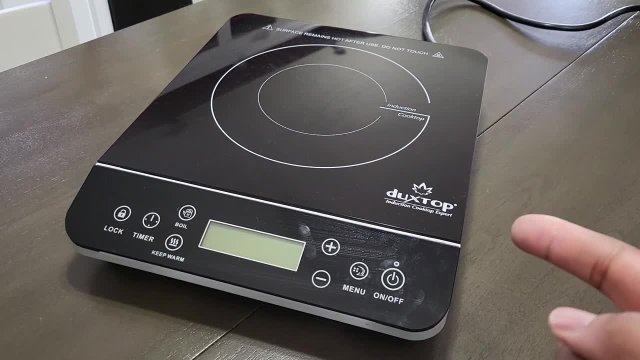 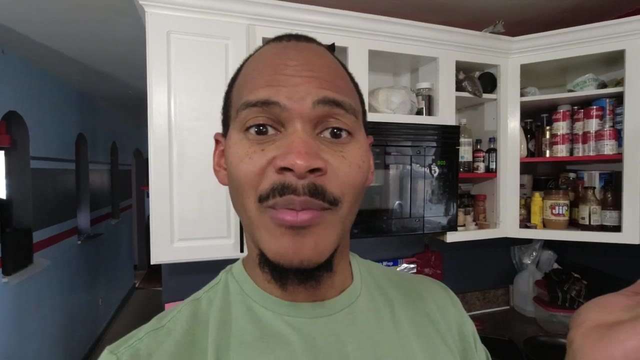 This Duxtop induction cooktop is said to have a variable wattage output, which may make it appealing for cooking on portable power stations. Let's get into this a little bit. What up I'm Ive? I like powering stuff from the sun, saving some coin in the process and being prepared for. 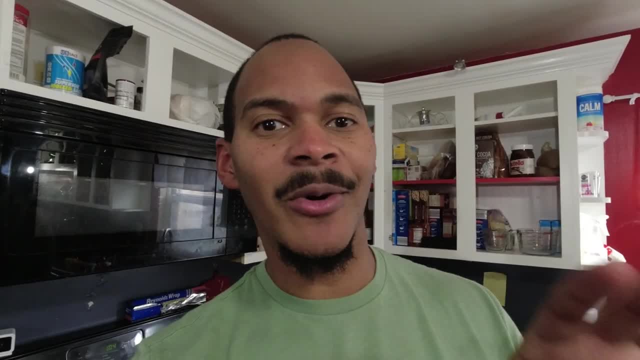 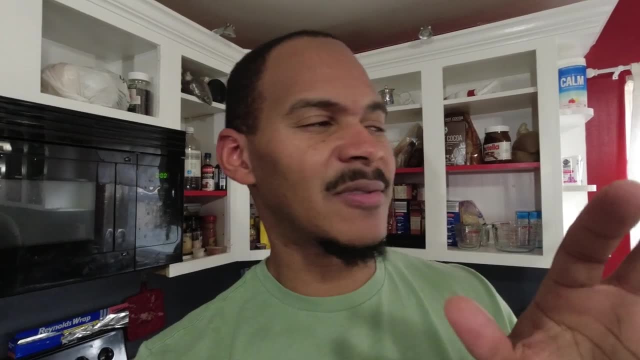 power outages: right, Right, I always wanted one of these little portable cooktops. I mean, way before I got into solar, I originally started with wanting the little coil one, and there's a whole reason for that that I won't get into, But just being able to cook during a power outage, or 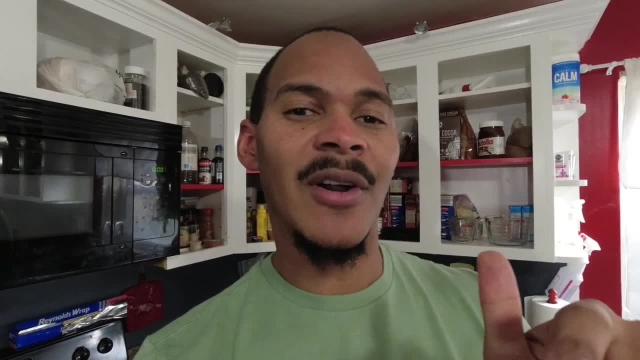 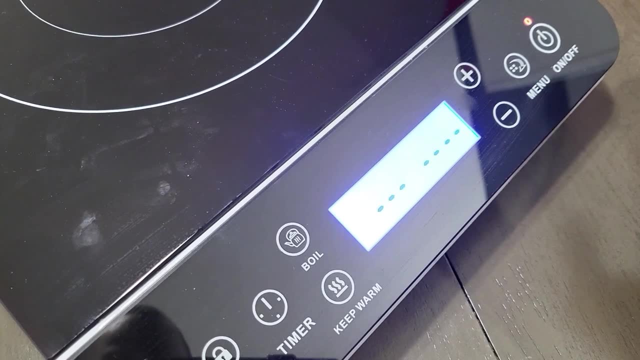 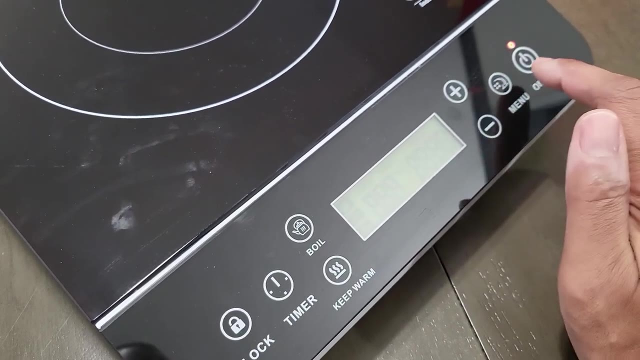 to cook out and about was really appealing to me. First, let's talk about some of the features. It has quite a few cool features. You have this nice display. I mean it's okay, It's not crazy. You hit a fan, turn on, I'm gonna turn it off for the sake of doing the video. It has up and down buttons. 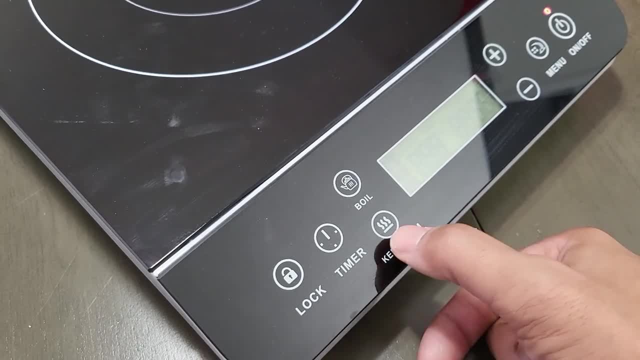 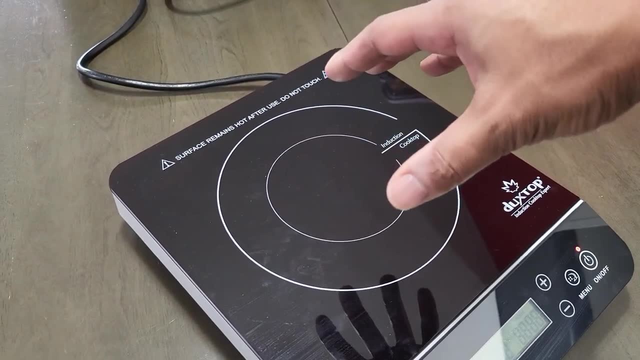 a menu button. It has a boil button where you can instantly do that- Keep warm A timer, which I think is really cool. It came in handy When I was using this to warm up some water with eucalyptus oil. Shout out to MJ who gave me that. 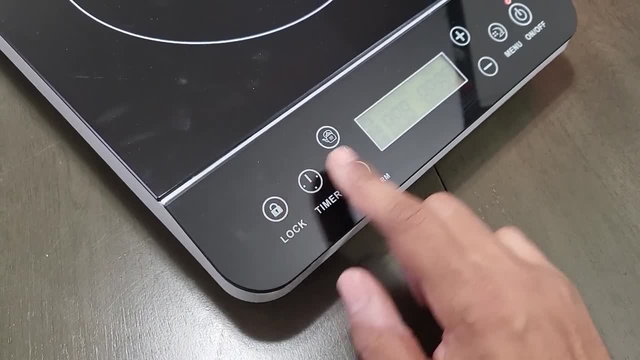 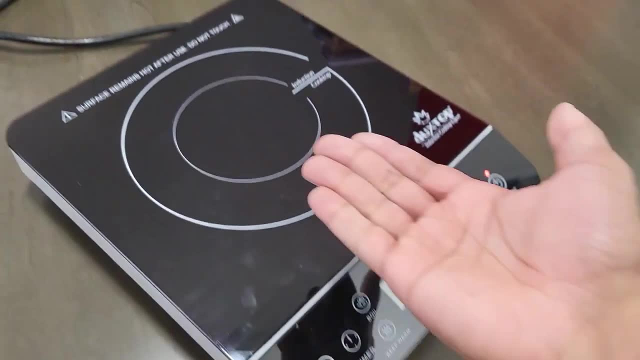 little tip. It helped out while I wasn't feeling well. And then there's a lock feature that stops you from changing these things, so no kids come along, or you don't come along and mess it up. I'm not sure you would want a kid around a hot joint, but whatever, It has a lock feature Here. 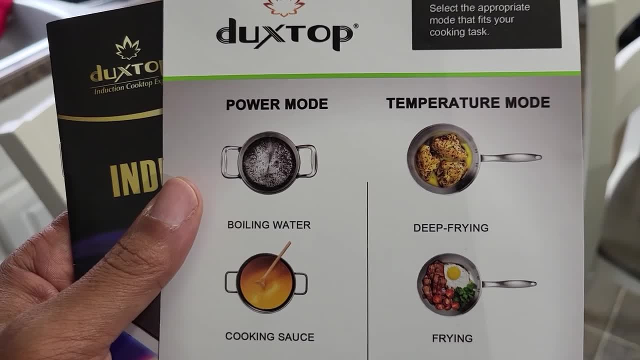 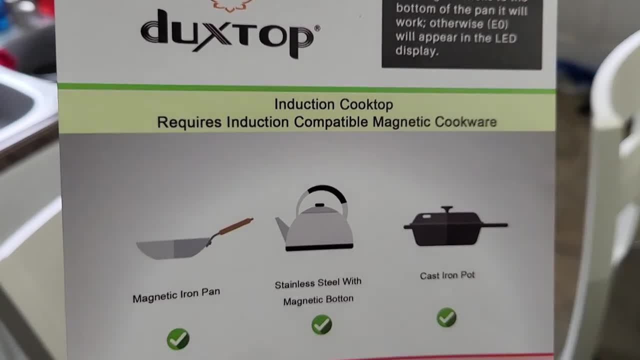 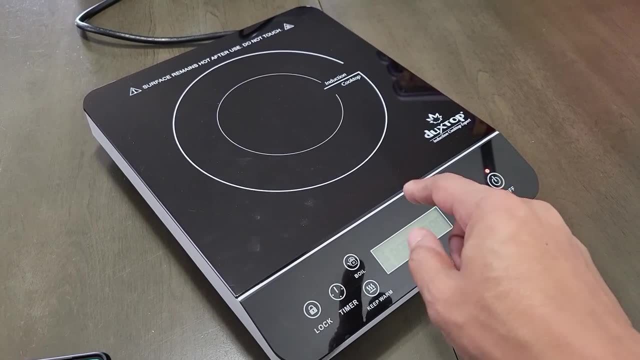 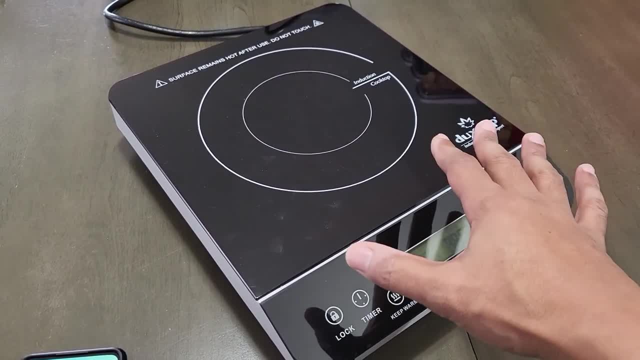 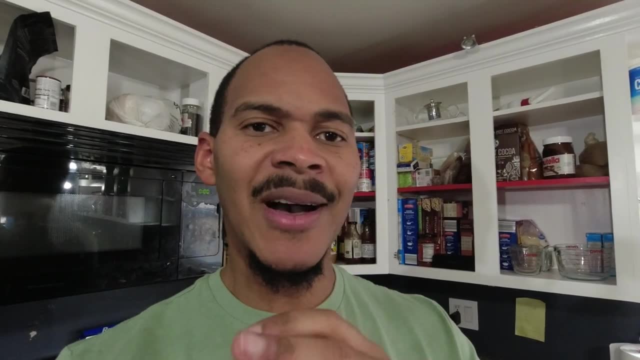 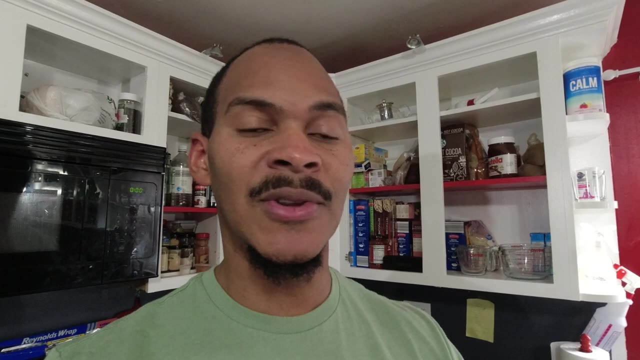 Wirecutter talked about the fact that this had a variable watt usage output, and it could go from about 100 to 1800.. Now why that's so appealing to me is because we have different types of power stations. right, You may not have a power station that could bang out the whole 1500 watts. 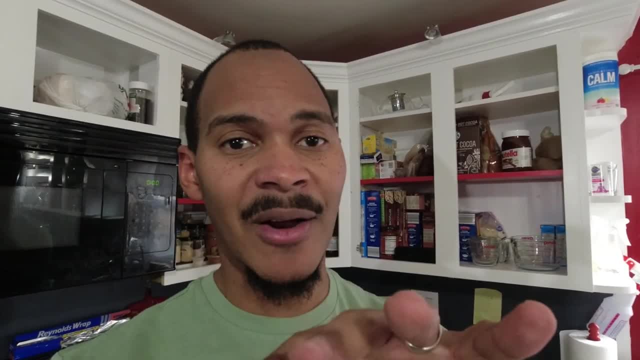 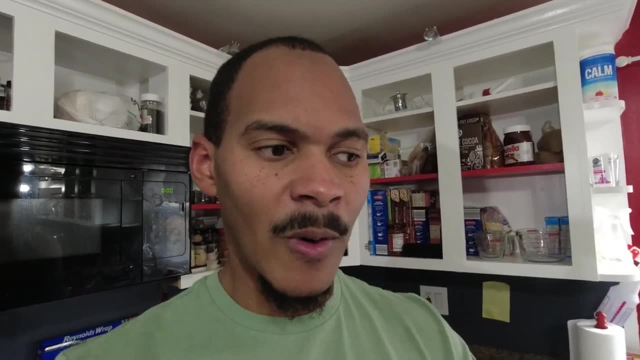 You may have a Jackery or something like that. We'll test some various power stations during the video, but I like the fact that it had a variable output. When I looked into induction stoves before, what it would say is it would have like an 800 watt, 1100 watt and 1500 watt. 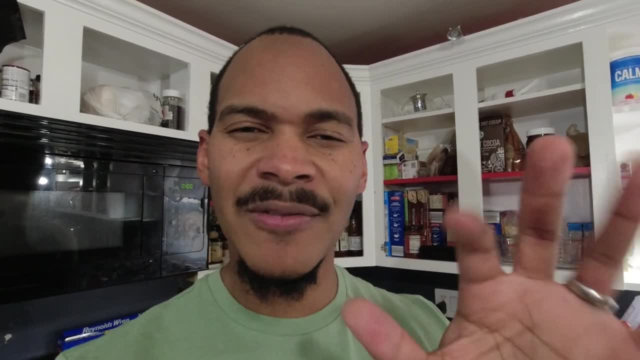 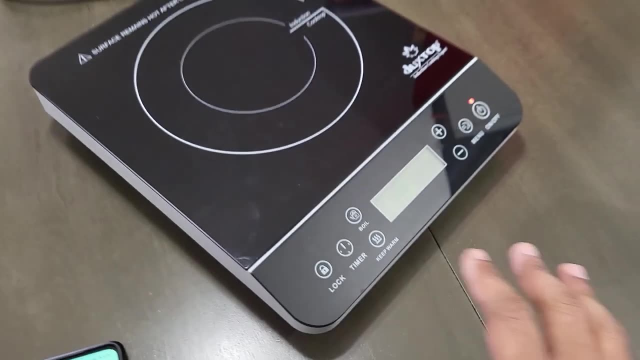 I feel like this one with its levels, should have some kind of variable output that you can adjust. We'll see how much that holds up, but I like the fact that they mentioned that. So let's take a look around the device. You can see the buttons are at the front. It has 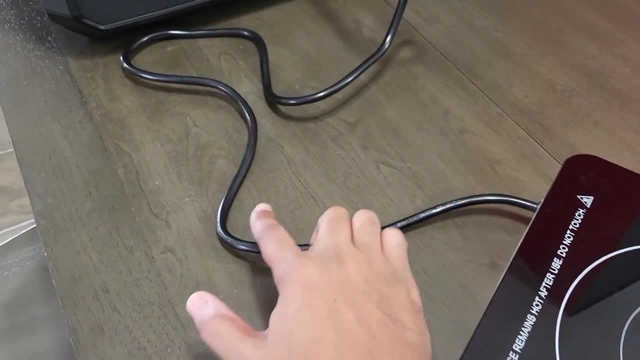 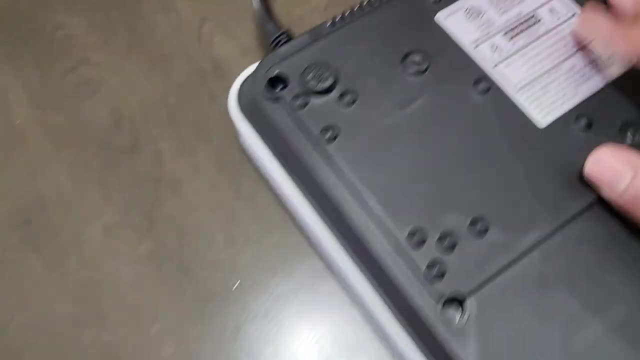 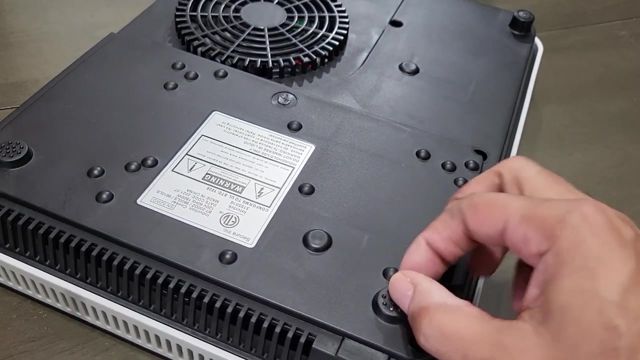 a very slimline form factor, super thick cable to put all that power through it, turn it over as a fan underneath and then we go around. there's not much else going on here. you just have the fan output over here. some rubber. they're not rubber, they're actually plastic feet that are built into. 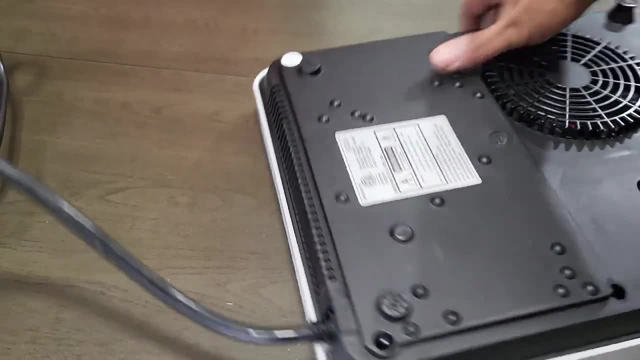 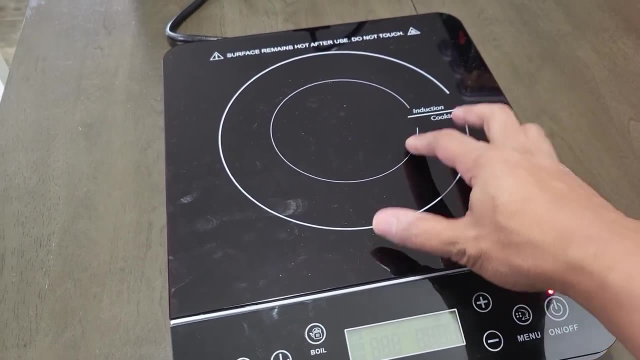 the base that give it a little lift up off of the ground and that's pretty much it. around the other side, we don't have anything else. when i first tried to use this, i would get an error, and what it does is it errors out if you don't have something that works with the stove on top. 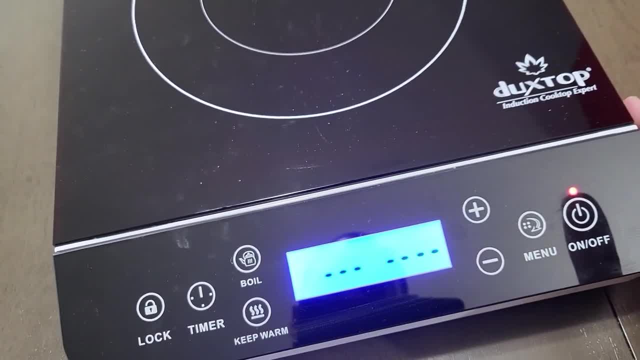 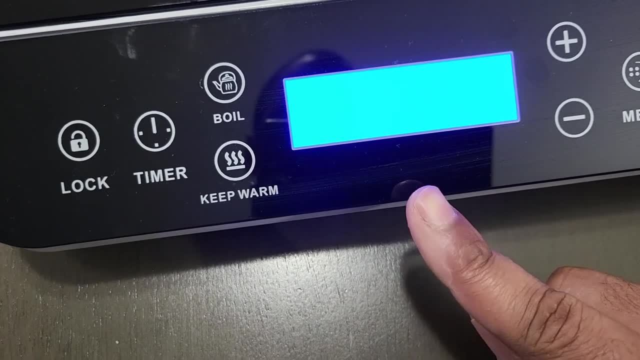 and then if you turn it on, you're gonna have to hear the fan for a little bit. if you turn it on and you have nothing on there, you can't do anything. you can't set it up, it just errors out like that. that's the same thing that happens when you have the uh pot on here. that doesn't work. so 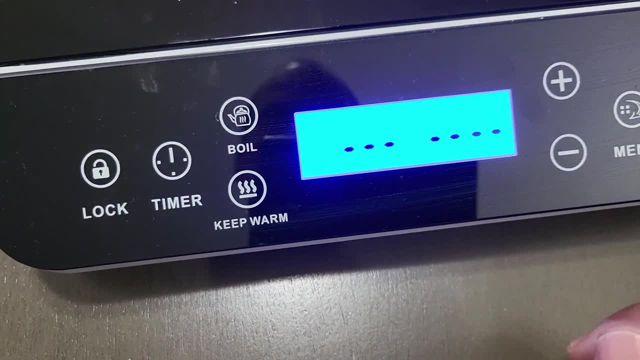 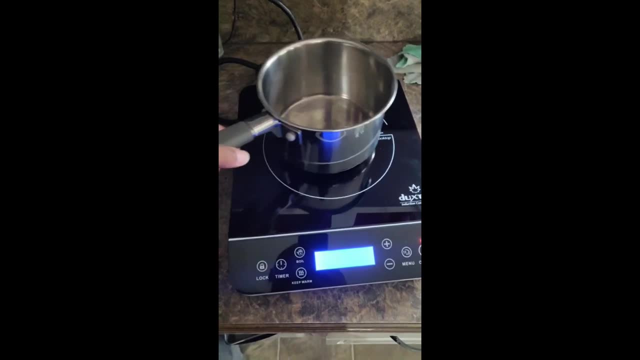 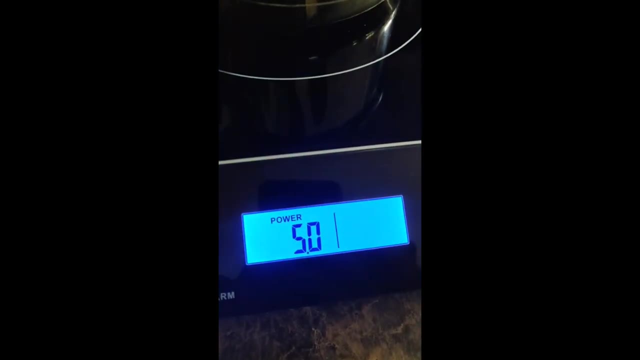 you can't adjust anything. i thought it was broken at first. i was turning it on and off and nothing would happen. so, sir, it appears that you are right. metal pot, drop it on. it sounds like the starship enterprise is beaming. something wayne coming through with the common sense. thank you, i turned it off and i was waiting for the fan. 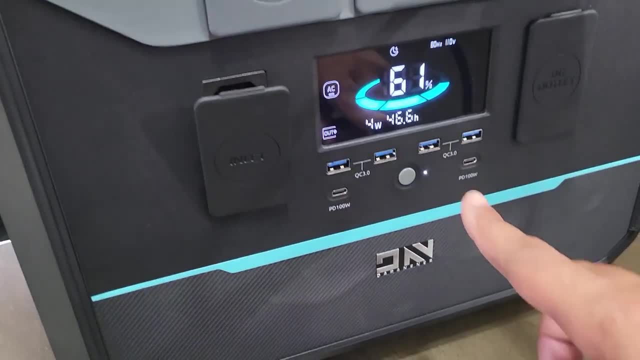 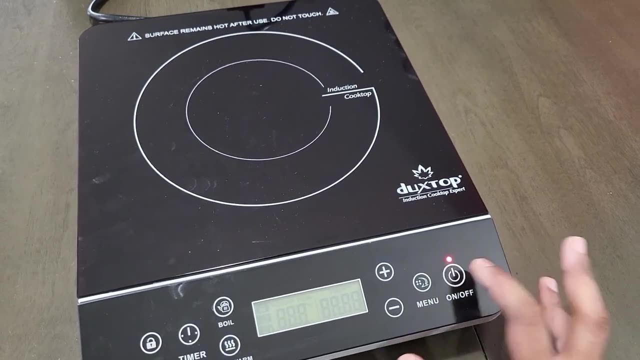 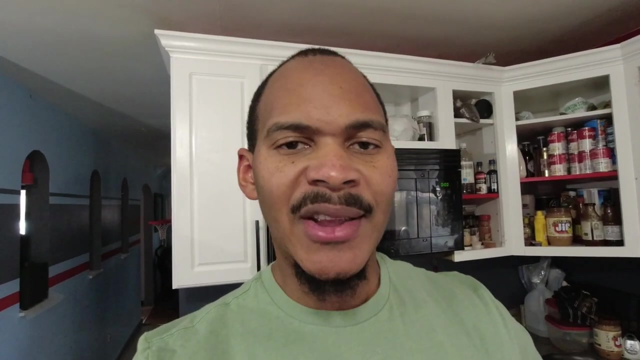 to turn off. but i'm looking at the duran duran and you can see it's consuming four watts with just the fan on, so that's pretty cool to know. i wasn't planning on recording it, so when you turn it on it actually went up to five watts. now we also need to talk about pots and pans joints that work. 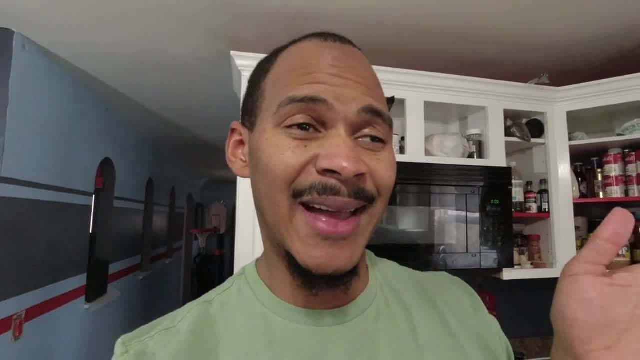 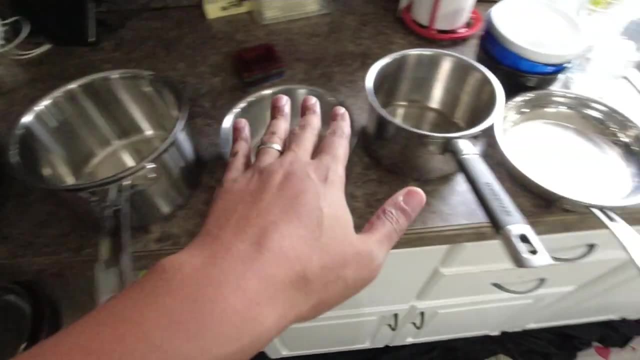 and joys that don't work. i have some pots over here so i can show you pretty much what's going on. here is what i noticed is these kind don't work. they're not magnetic and these kind do. and how i tested that: i just grabbed some magnets for my kids toy set and that kind of goes. 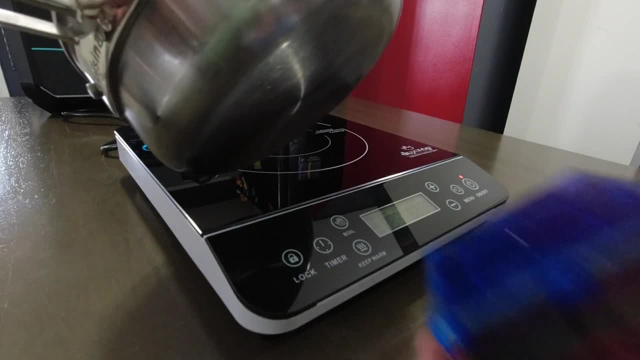 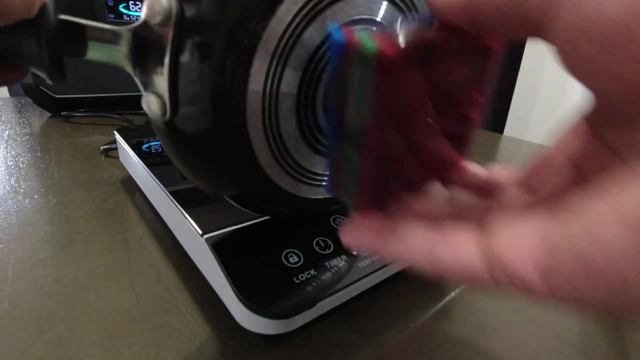 on. um, actually, let me show you a bit better. i basically just grabbed my kids stuff and put the the bottom and see if it was magnetic. you can see that these are it sticks. and then when you grab something like this, you put the magnet on the bottom- nothing. so now i have placed the pot on. 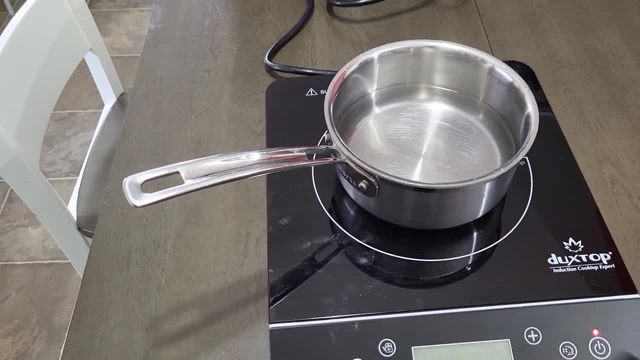 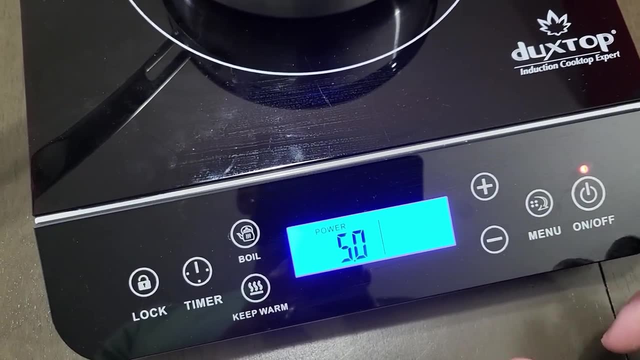 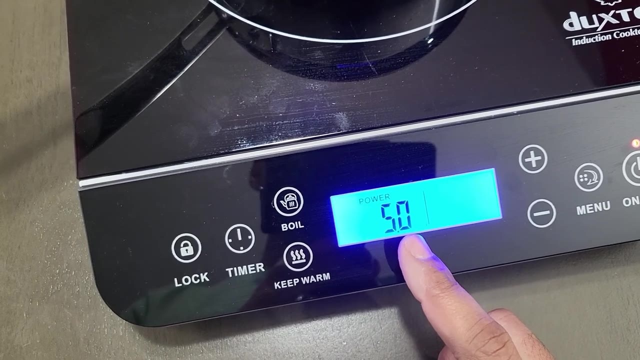 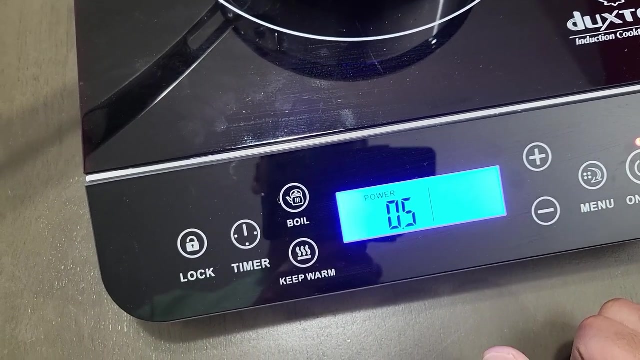 top. it has about, you know, an inch of water in this little, whatever quart pot it is. i'm going to turn the device on and then, now you see, you hit menu, it starts out at power level 5.0. now i don't know if that has a correlation between the watt usage, but it can go down as low as 0.5, and 0.5 is actually. 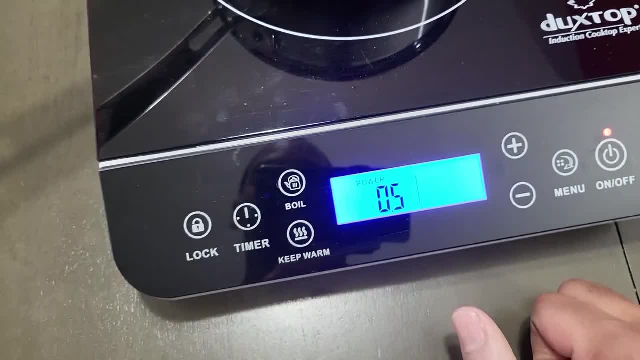 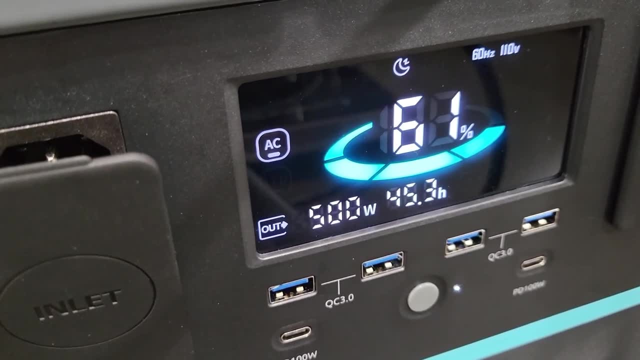 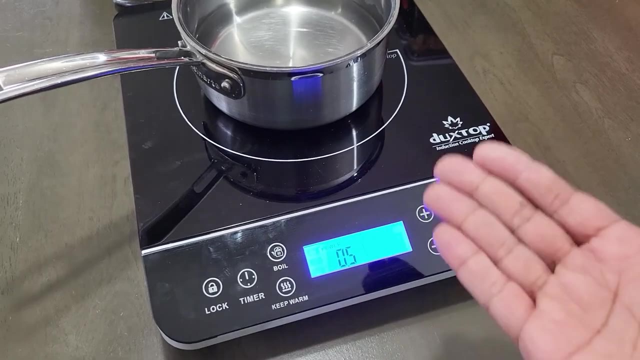 doing what i would presume is nothing. i'm watching the output over here and it's saying: five watts, oh no, it just kicked back up. what it seems to be doing is heating up to a 0.5 power level, which is not much, so it doesn't stay on it just. 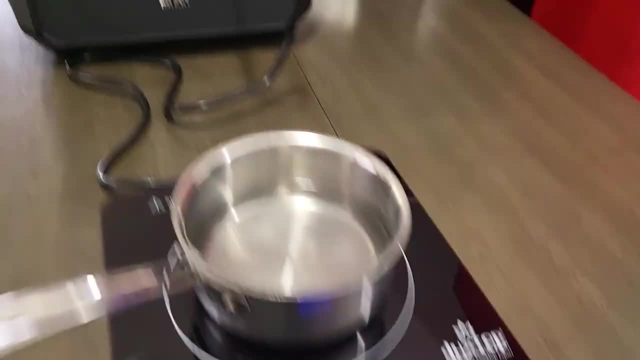 you can see that it's heating up to a 0.5 power level, which is not much, so it doesn't stay on. it just kicked back up, back on and it went back up to 500 watts. so let's toss it up to, let's say, 2.5 and see what happens. 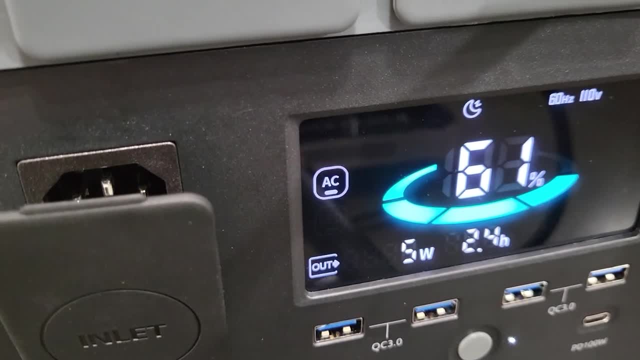 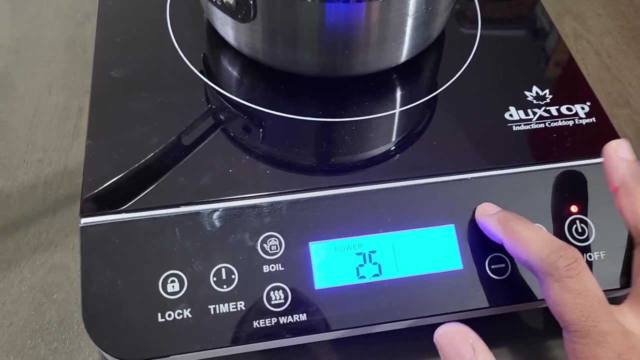 so over here we have about 700 watts that came through. so instead of kind of dealing with this intermittent heating capacity, what we're going to do is we're going to turn it all the way back up to 5.0, because that that's where it defaults from, and then i'm gonna let this sit for a little bit. 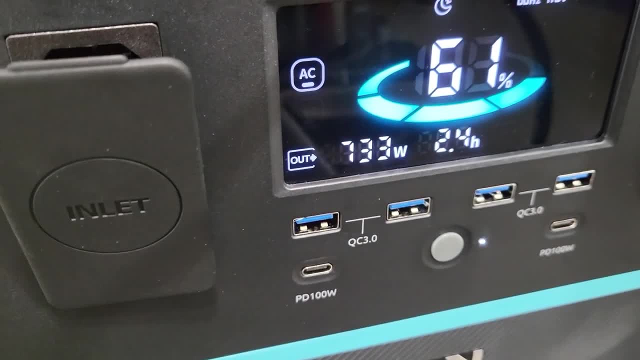 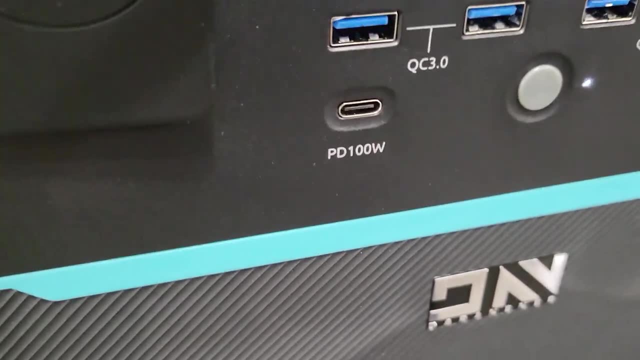 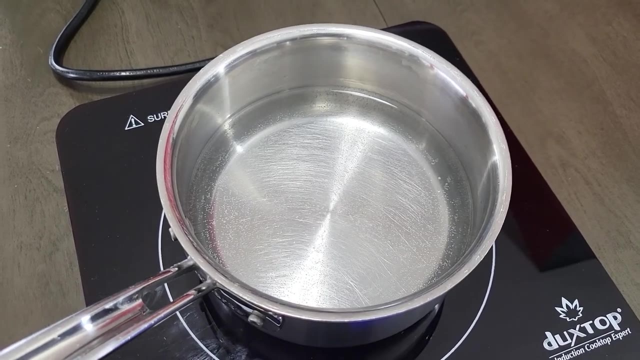 and see what it actually does if this power draw stays there because it's trying to maintain a five level. so you see 700 watts. dang shakycameracom. so that has settled in real good. one thing about induction stoves is they're really fast. 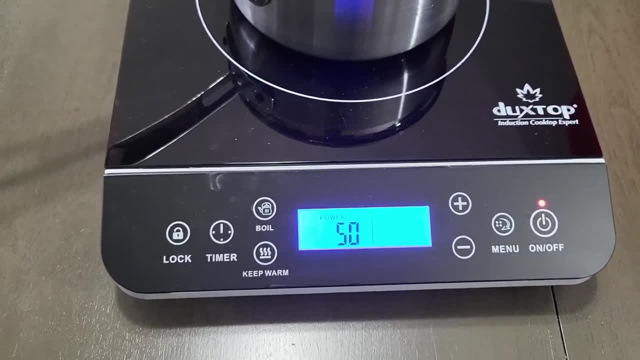 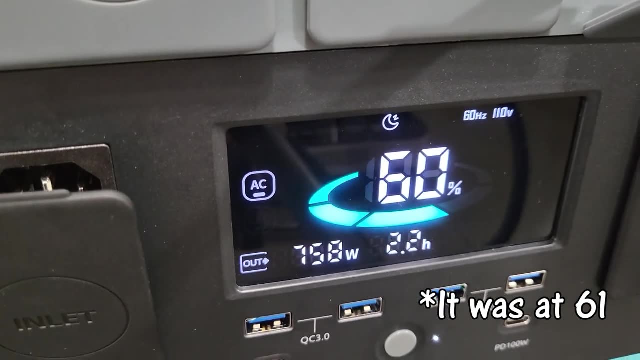 this has only been on for maybe about uh, what you can see it's still at 60. if you pay attention to the percentage before, it's using about 700 watts and this is almost starting to show bubbles. so let's go ahead and turn it on and see what happens. so let's go ahead and turn it on and see what happens. 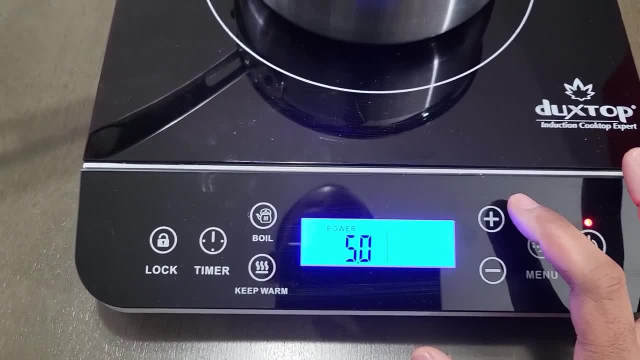 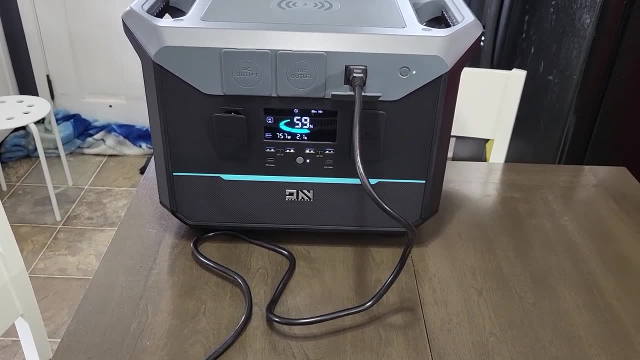 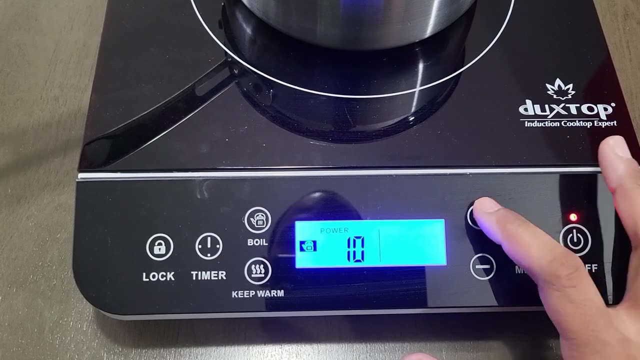 ahead and just turn it all the way up to its highest setting, see how much power we draw and see if the duran duran can uh handle that draw, because it's a 2000 watt, 2000 watt hour device. this one is rated at as high as 1800 watts, so we're going to go power all the way up to 10.. 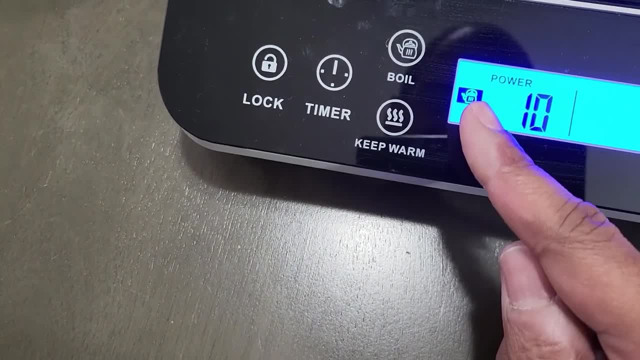 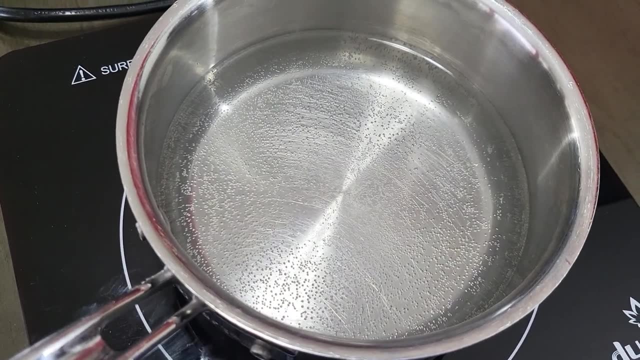 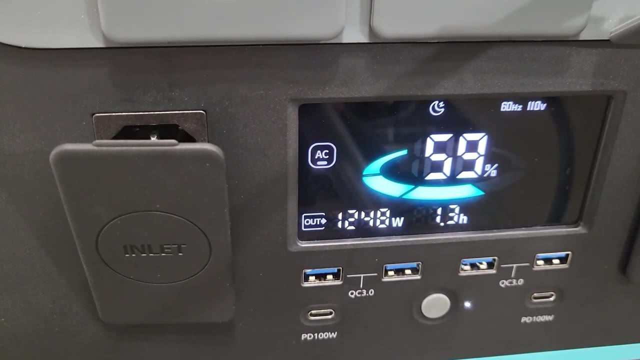 10 is the highest it goes. you can see, at 10 it has that little icon and that's the boil icon. i'm going to keep this going live because you can see that these bubbles are starting to form and i'm looking at the duran duran and it's using 1250 watts. 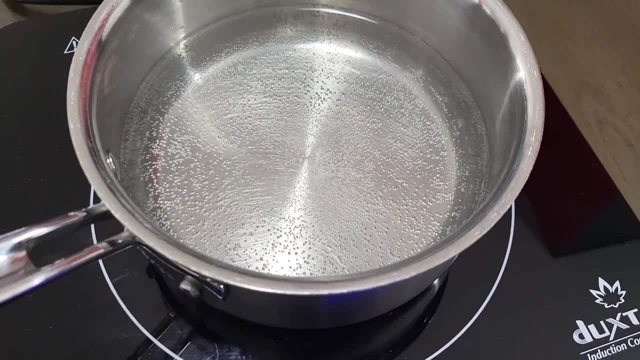 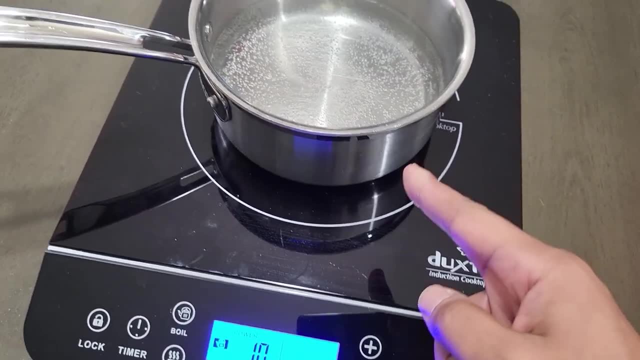 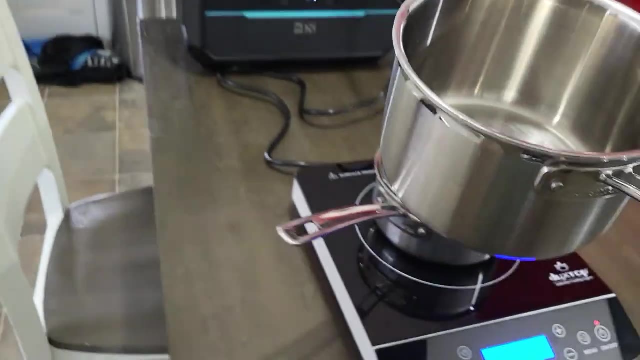 so this is pretty fast for an induction cooktop and it's not using nearly as much power as it's rated to use. i wonder if that has something to do with the surface area that we're using. i do have maybe a bigger pot. is this pot bigger? yes, a little bit. no, it's about the same. 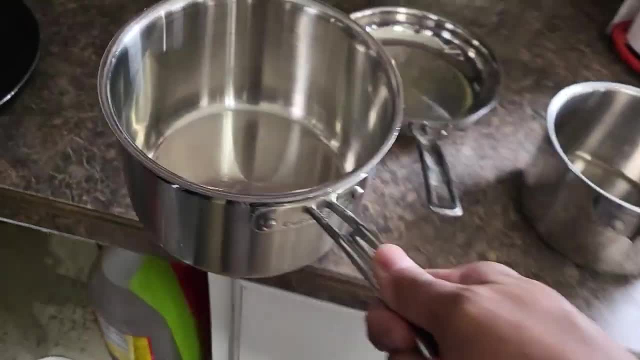 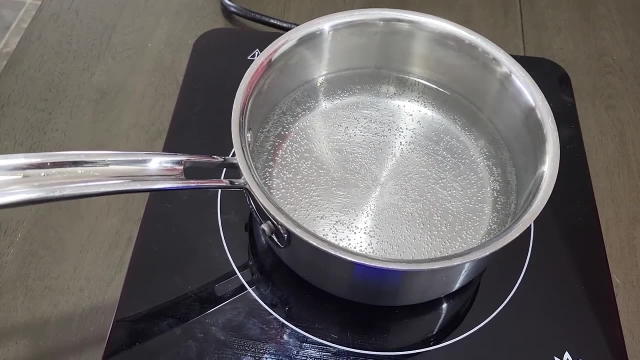 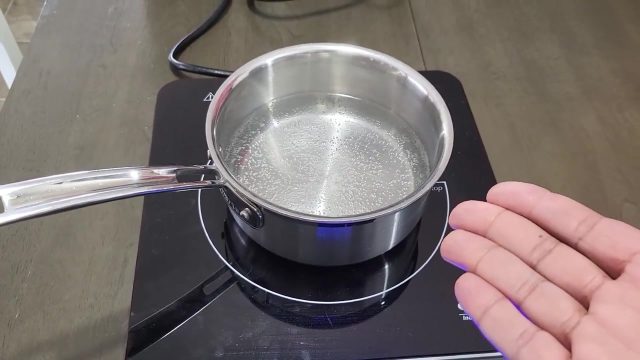 size. it's not that much bigger. i don't have a bigger pot that i can use on here. i've kept this clip going live. it's a minute and 40 minute 30. and you can see that water starting to boil now. this is useful because in a situation like this, you don't want to be waiting around. 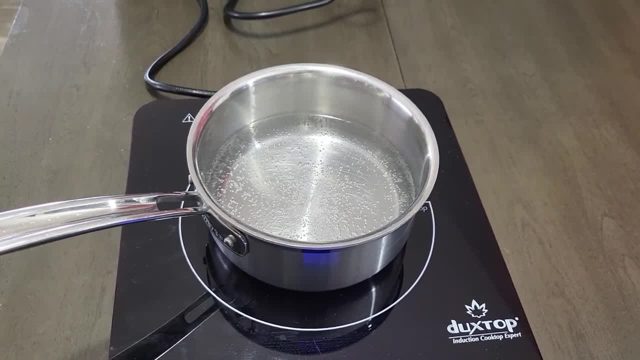 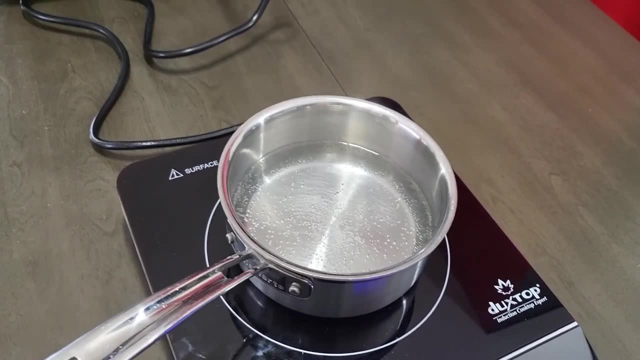 ready to cook. so the fact that this can kind of get going really swiftly. boil your water for your coffee or whatever you weirdos drink when you're out in the woods. i say that with love. y'all know i love y'all woods people. i ain't that still using the same amount of. 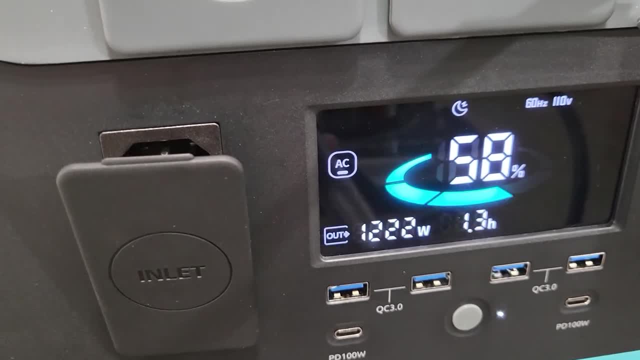 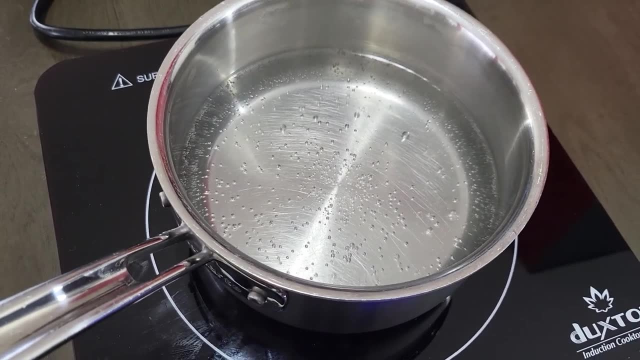 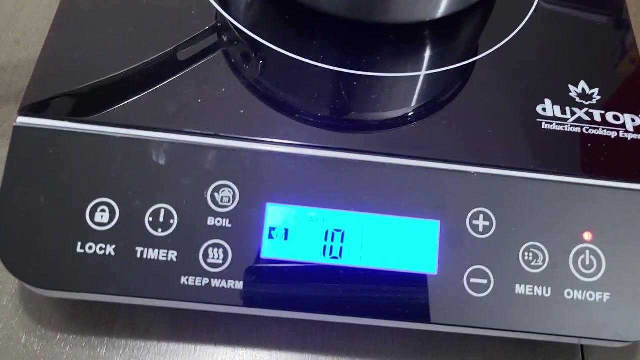 power about 1240 watts, and the party's getting started. i would say in another 30, 45 seconds, maybe not even this water is going to be boiling and this is at the highest level it can get on the level setting. i stopped recording by means of habit, but i literally just turned the recording. 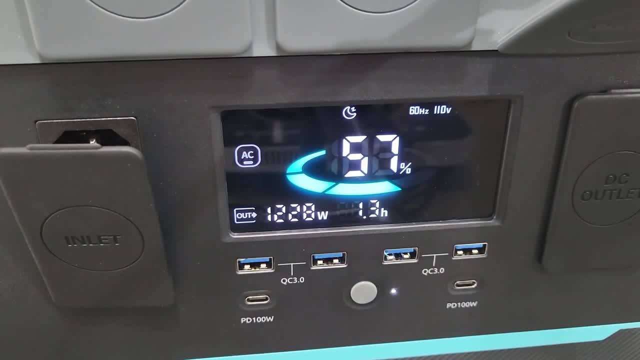 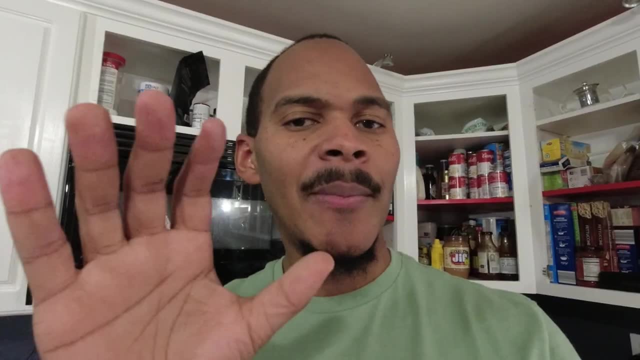 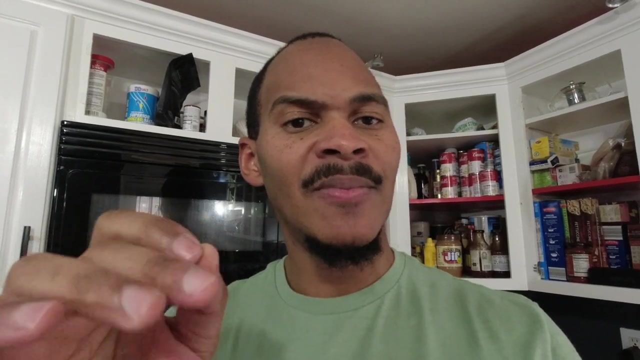 back right back on. you can see it's at 57 and still showing 1200 and some odd watts, and this water is pretty much at a rolling boil. in this video i'm not going to focus on the idea of time to boil water and all that jazz. i'm mainly interested in the feature set and how much power. 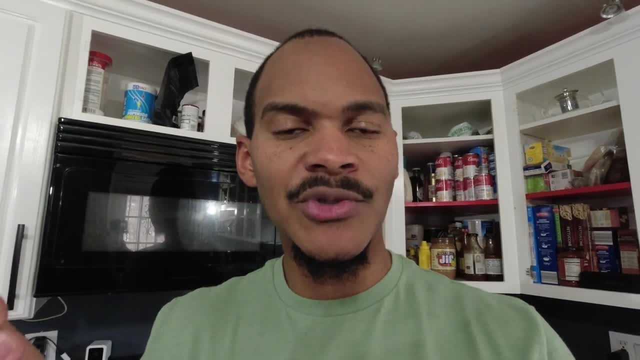 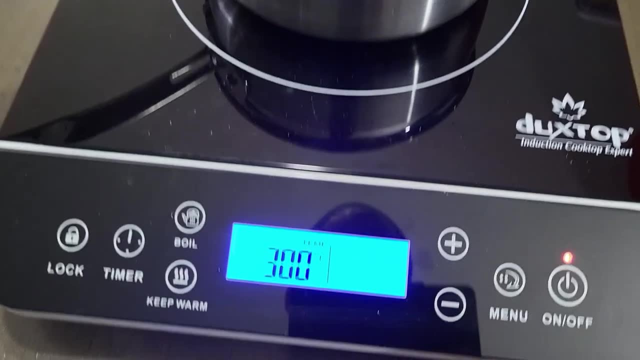 it uses, so that you can understand what kind of power station you can use this joint on and what you can accomplish for whatever your needs are. and then also in your menu you have temperature that's 300 degrees. now, that's interesting. let's put an empty. 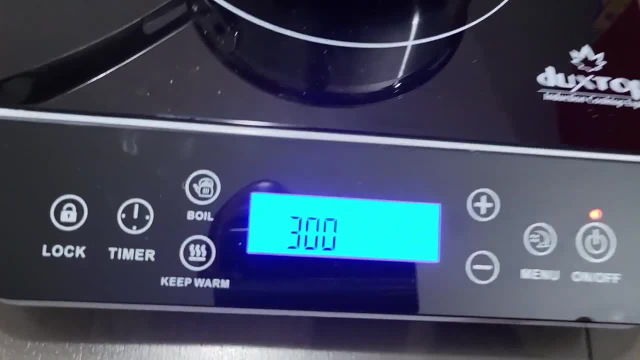 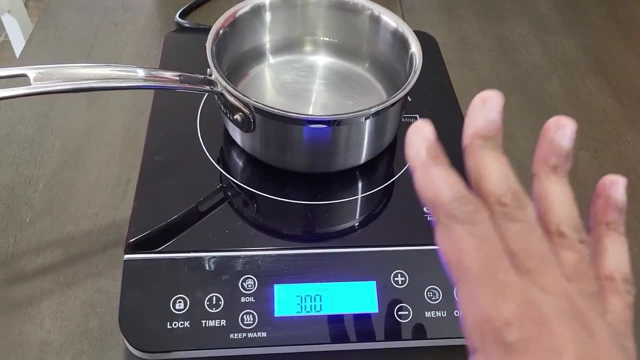 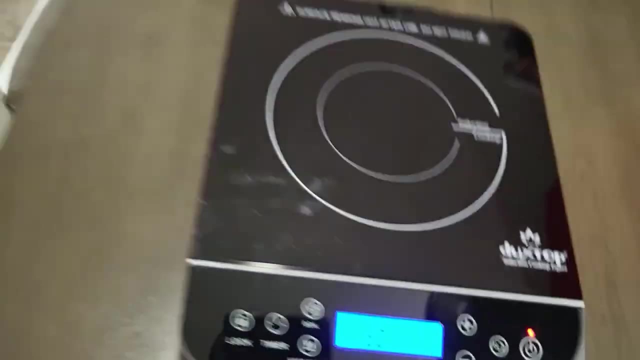 pot on here and see what this does, because at 300 degrees it's using about a thousand watts. i don't know how useful that information is to me, but i'm just kind of going with the flow here. see that i took the pot off. we got the error. let's bring this pot over here. 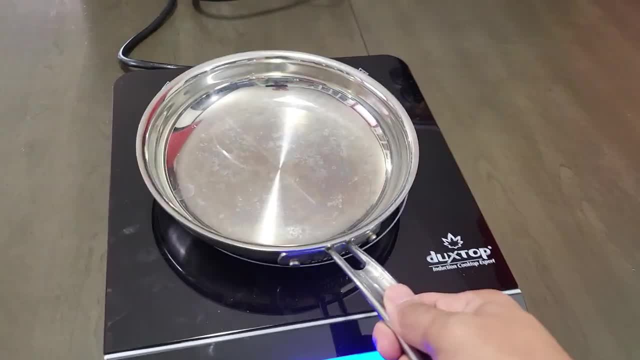 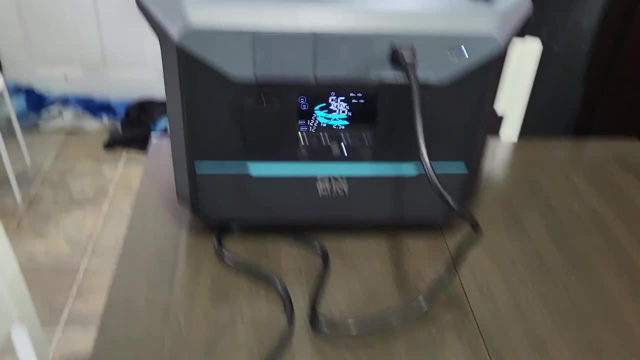 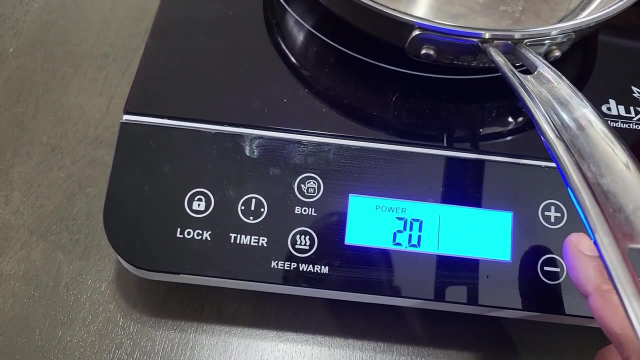 let's just put- let's do the saucepan back on. you can hear them: enzymes. it did a pretty good job: jump right up to 1200 watts at the 300 degrees. now i want to get out our degrees and go back to the lowest power setting, which is 0.5, and let's see what 0.5 does when it kicks in. 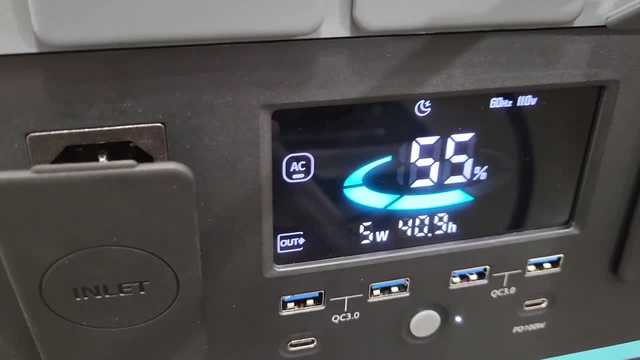 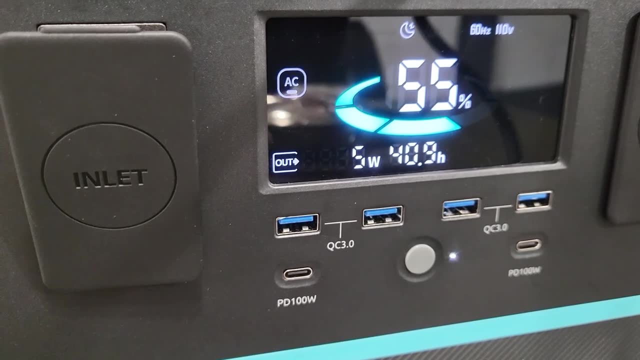 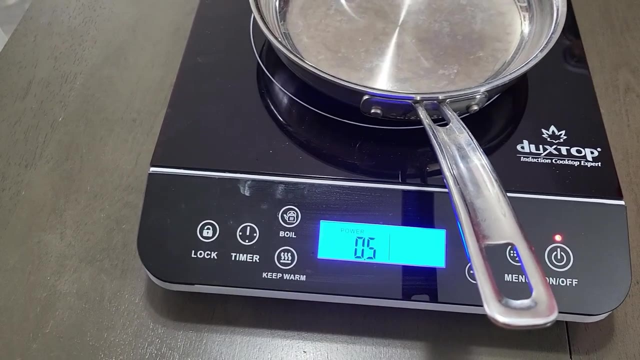 if it kicks in okay. so it kind of used about 400. i don't know if, based on the 0.5, the power zone, that you can use as little as 200 watts, 100 watts, i don't see that. now, if they want to play the numbers game and 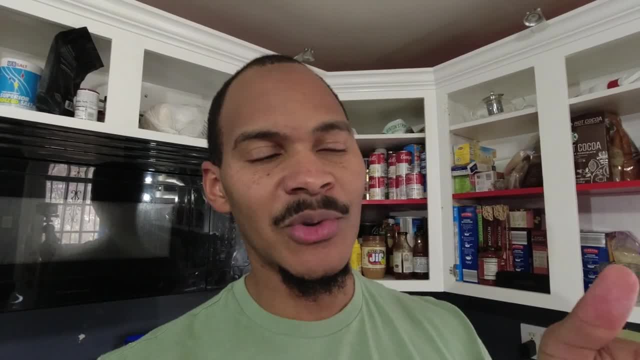 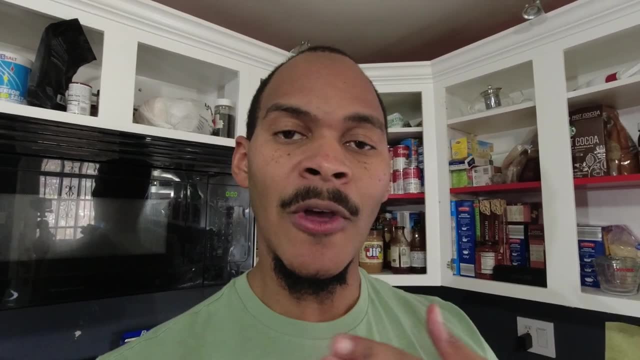 do well. cumulative power over the hour equals to 100 watts. i respect that. that's not necessarily the most ideal thing to base it on, because with us in power stations we're going off of how much power we're going to be using and how much power we're going to be using, and 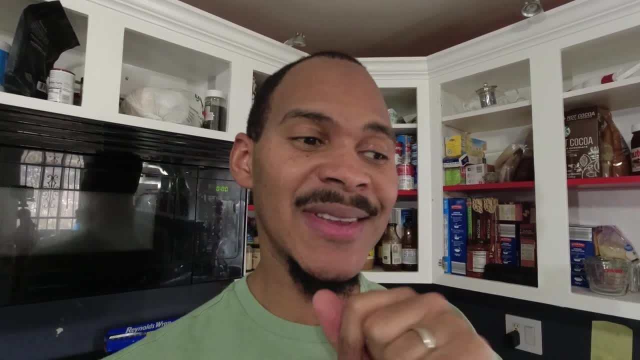 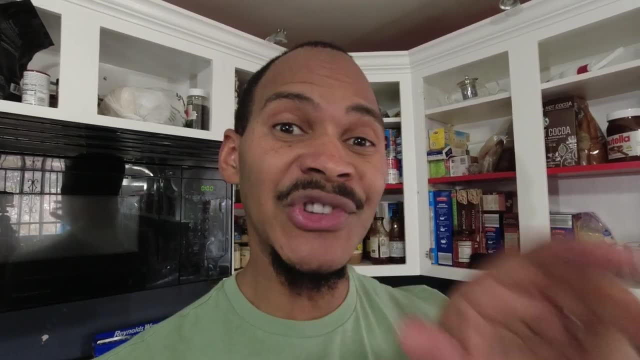 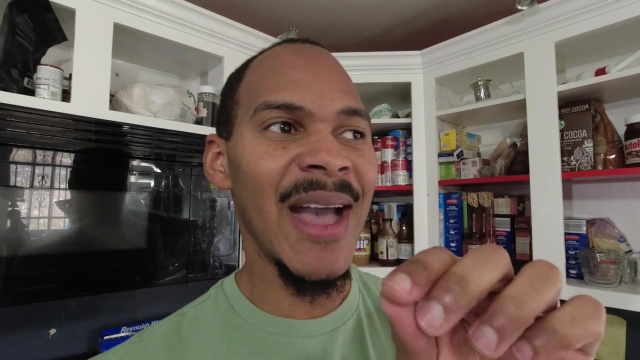 how much watts our inverter can push. now, interesting thing: you know you have the eb3a, the eco flow river max, the eco flow river base, the eco flow river og model that have what's called x boost. maybe i should try that on one of these. i'm gonna try that. you see what x boots does. 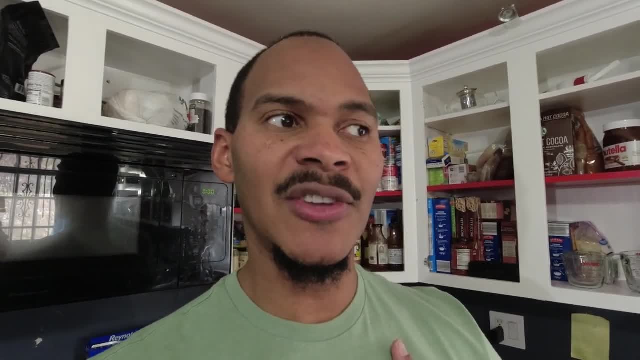 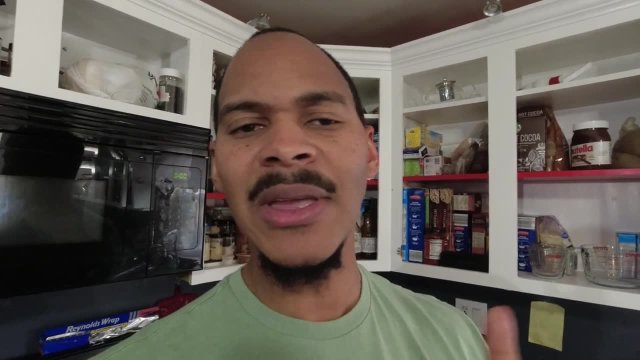 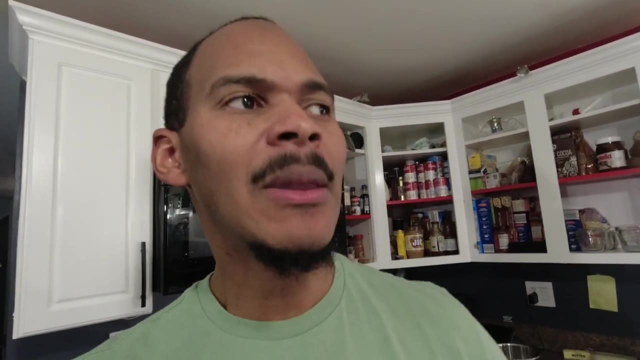 because my understanding is you should not do that on sensitive electronics, but things that use heat you can. so i think i'll use the eb3a because my eco flow river is not charged, because i'm thinking about the watt usage. well, okay, let me take all of that. 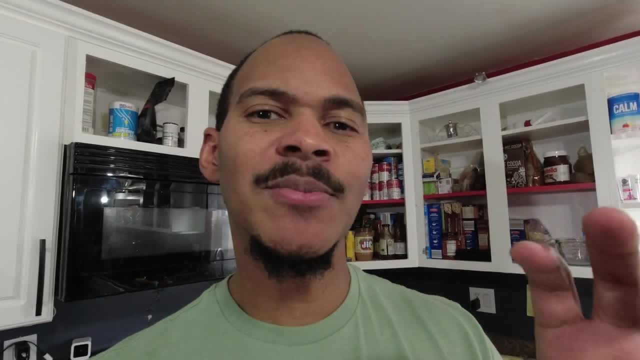 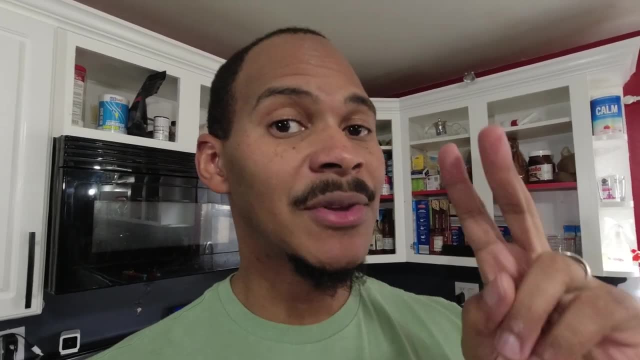 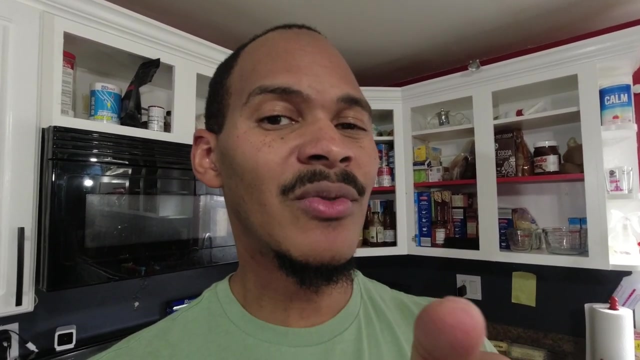 back what we have with the x boost feature. the x boost style feature is the fact that we can get these induction stoves to go to a higher temperature. but the eb3a is supposedly rated to 300- 600 watts on the inverter. i believe the base model river is 300 watts, which is 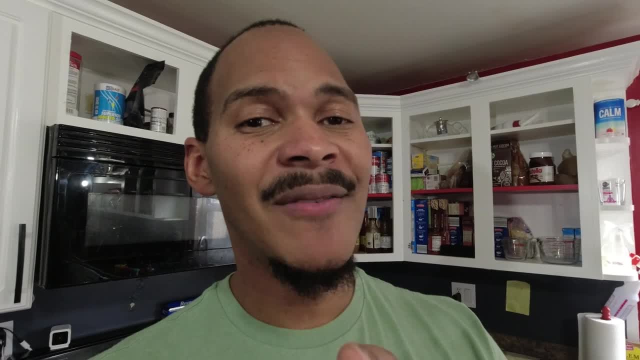 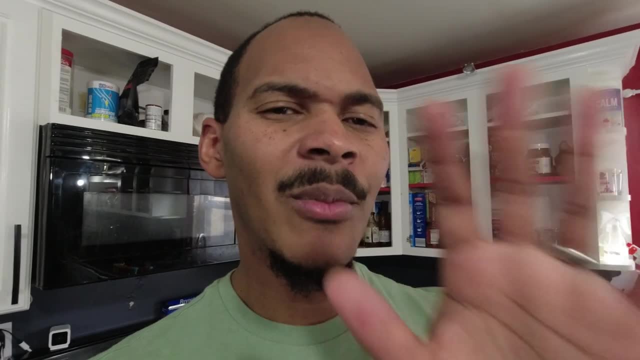 yeah, the river max is 500 watts and then on its x boost it doubles to a thousand. anyway, i feel like i'm rambling. let's let me figure out how i'm going to test and what i'm going to do here, to give you guys. 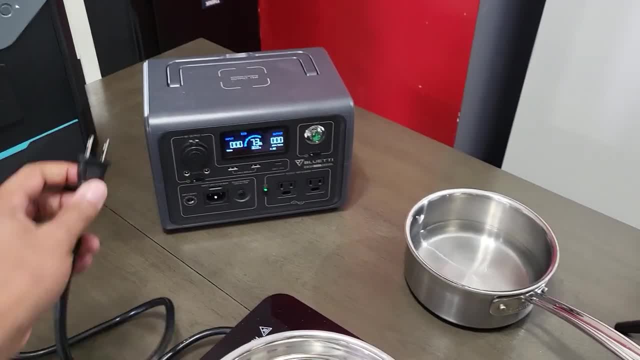 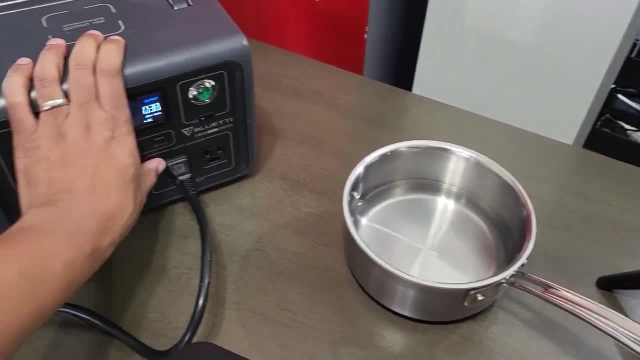 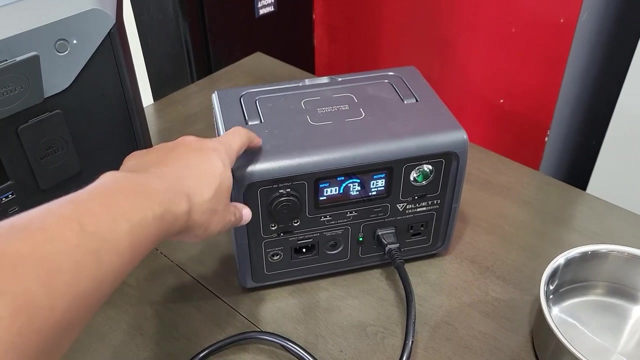 another example of using this on a power station. now, what i have here- blue eddy eb3a, i'm going to plug it in the uh inverter- is already on. i will tell you, guys. i tried to use, i believe, this on a heater that supposedly only does 500 watts and this failed. i don't have footage of it. 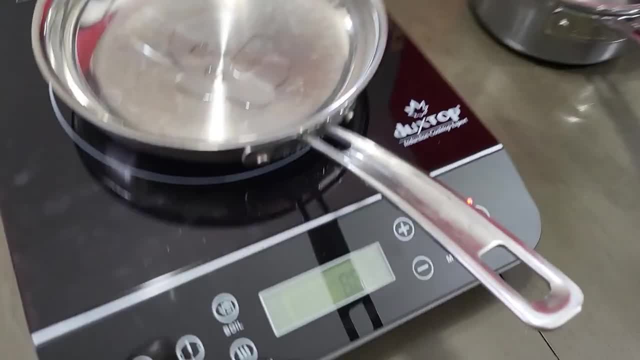 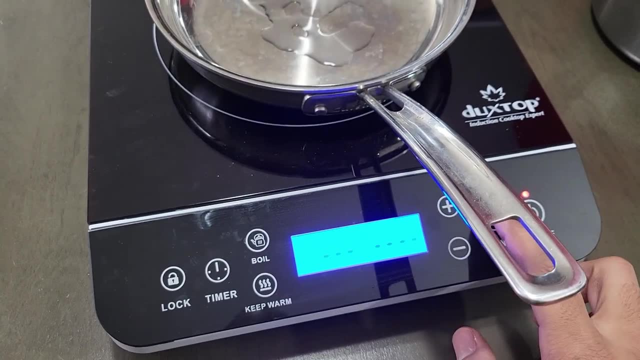 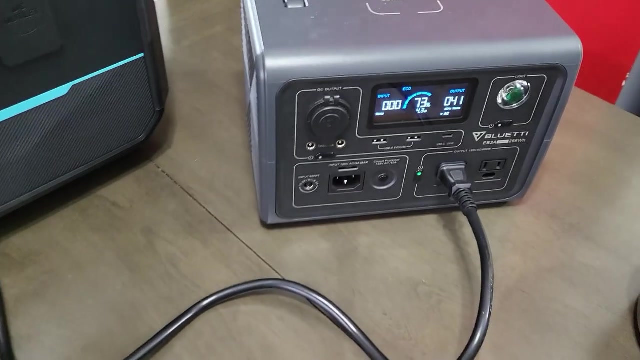 but it was my experience, so let's turn this on. you notice it's going to start at the five level. i'm gonna drop it all the way down as quickly as i can, so i'm gonna do this live. i'm not gonna cut away. let's watch it. 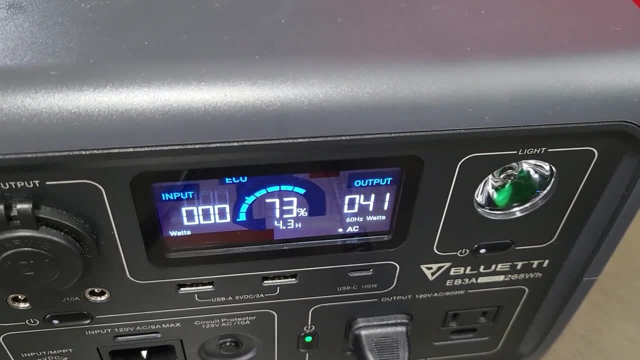 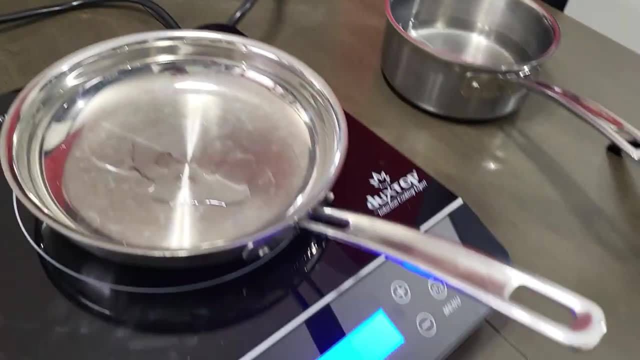 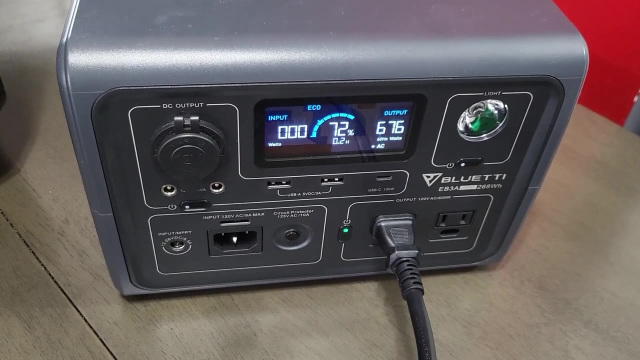 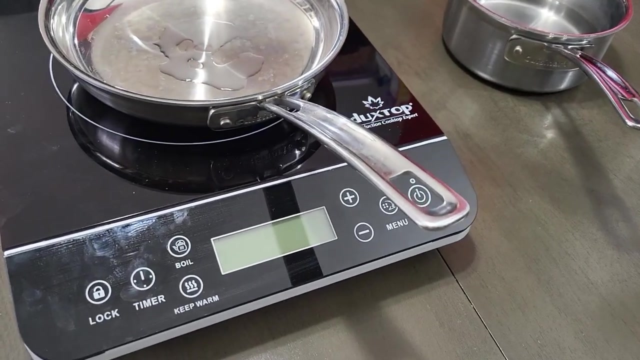 output goes up to about 546 and it's doing that just fine. let's push it up a little bit. let's do maybe 1.5 jumping. oh yeah, it was like six something. you bugging, fam, it's pretty cool, okay. next thing we're gonna turn on the boost feature of the eb3a and see what it does then and shout out to hobotech. 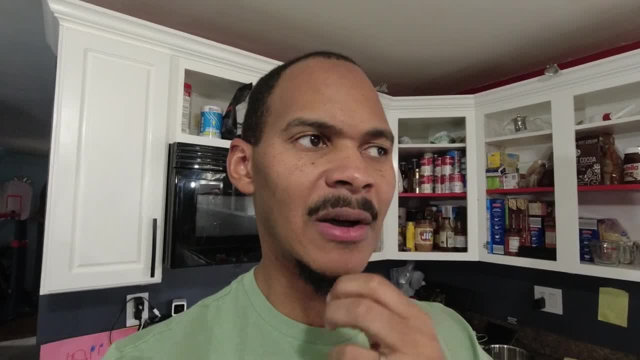 because he's the one who's going to be doing this on a power station, and he's going to be doing this. and he's going to be doing this on a power station, and he's going to be doing this on a power station, explaining what these boost features, uh, perform. what they do is they lower the voltage, so that they can keep the amps at the amount of power that the device needs. so you may end up with 90 volts, 81 volts, and that's why sensitive devices can't use this feature, because that voltage variance going, dropping down that low, could cause problems for the device because it's not getting the 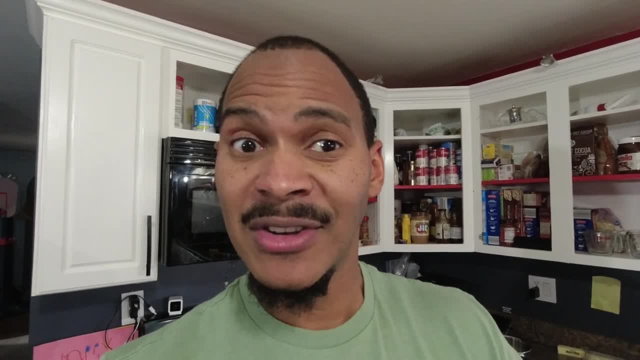 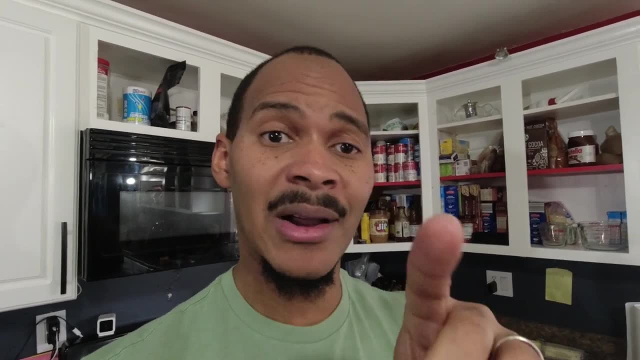 voltage that it wants. but they say: with induction loads, induction cooktop, right. they say with an Induction loads that you can use the X boost. but y'all, tread carefully, I don't use X boost, I'm just doing it for this situation. I have never used it ever, ever check this out. 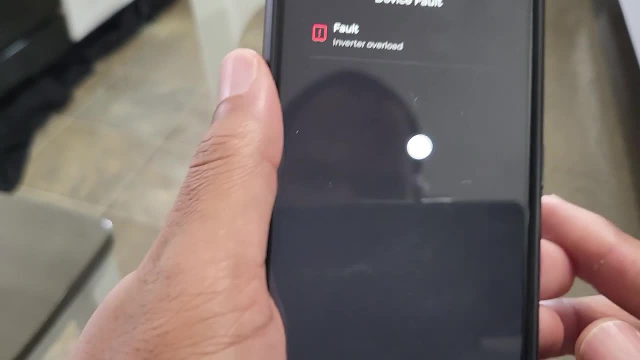 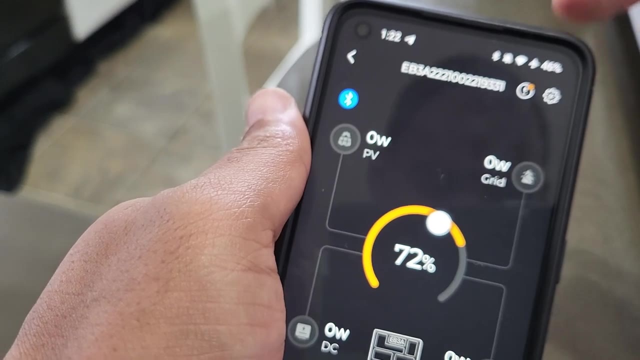 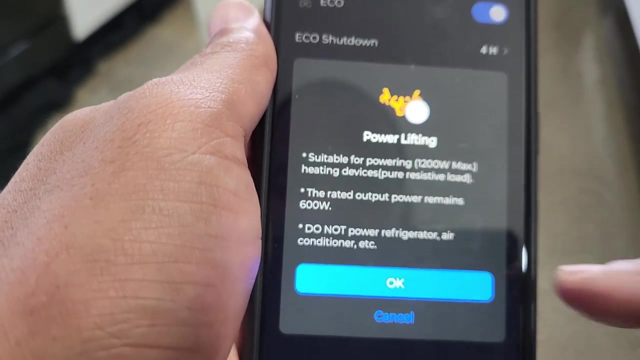 it actually shows in the default details what happened. so it's a Inverter fault, and that was right here up on that little Exclamation point. so now let's go to settings- Power lift- that's what this is called- And then it gives me a warning: suitable for powering 1200 watt max heating devices. 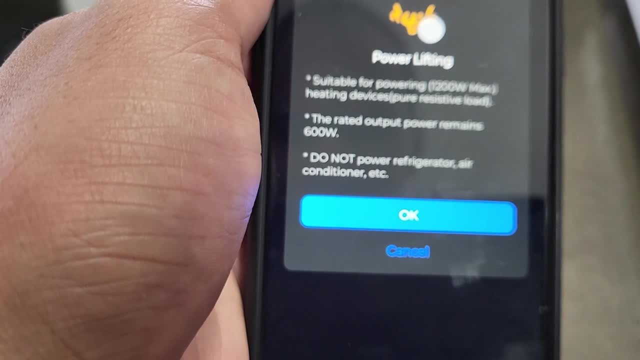 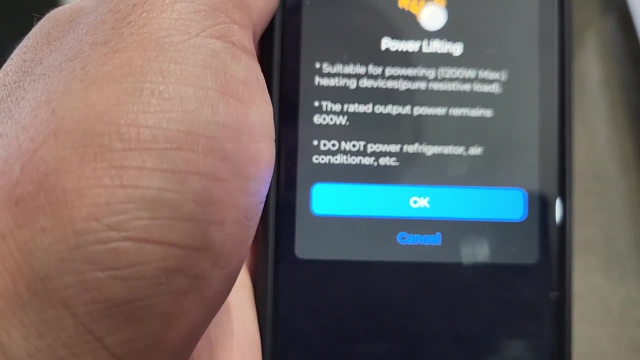 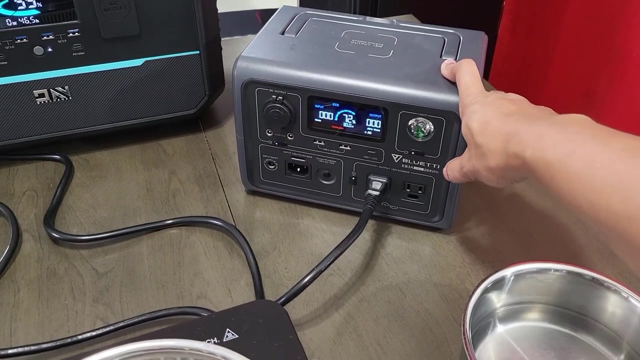 So it specifically says heating devices. the rated output returns. the rated output power remains 600 watts. do not power refrigerators, air conditioners, etc. there you go. power lift mode is on. Device is going back on. it still has a fault. the AC light is blinking. I 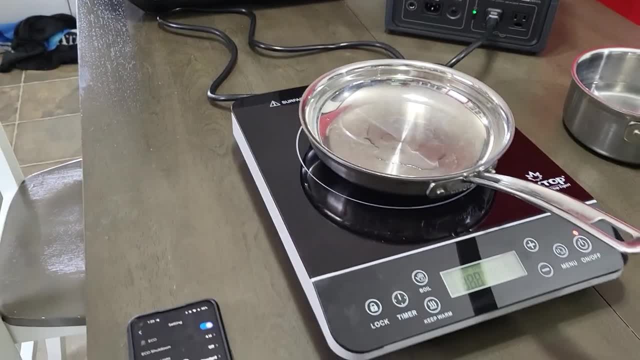 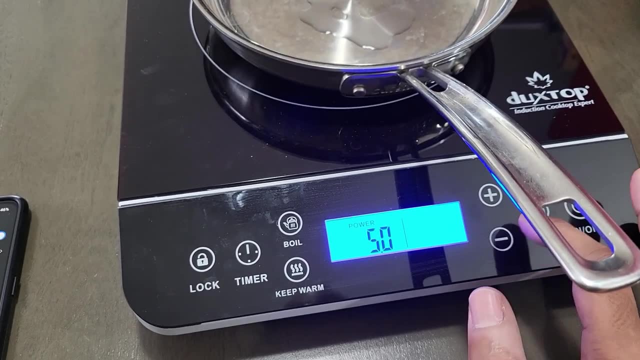 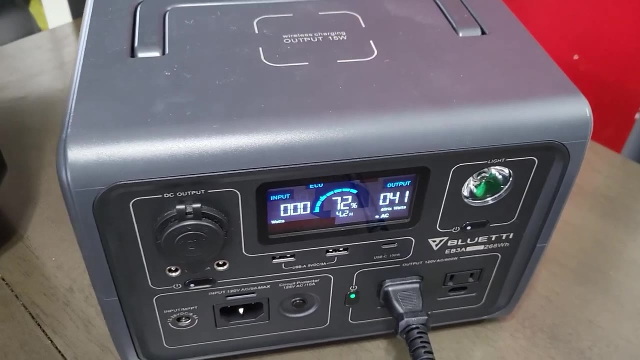 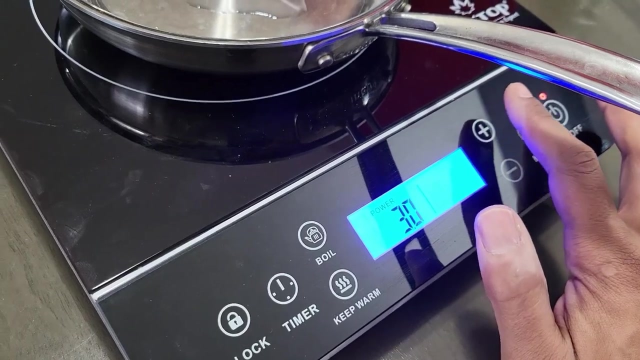 Just held it and then it turned back on and Now let's do boom and Let's drop it all the way down again menu: All the way down to 0.5. It was doing 500, So we'll bring it up to whatever we did before, which I don't remember. let's do 3: 3.0. 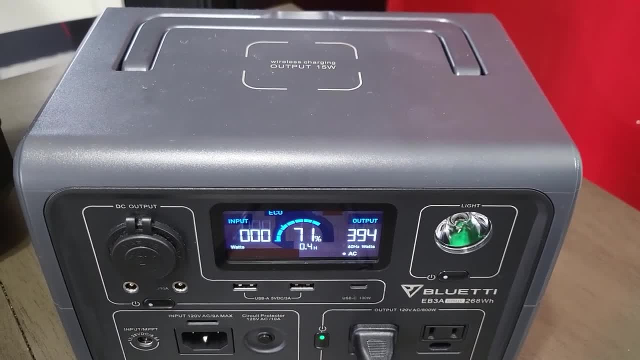 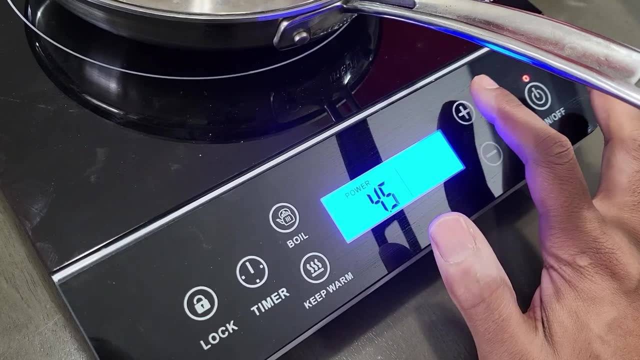 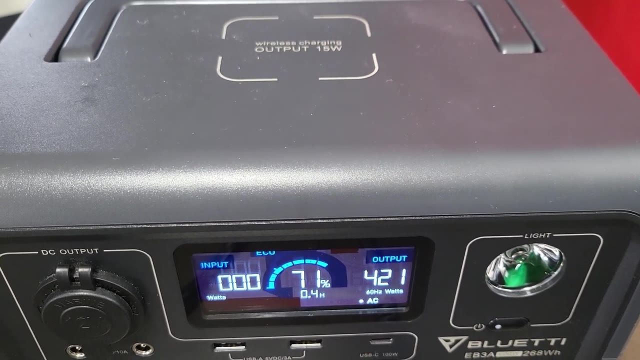 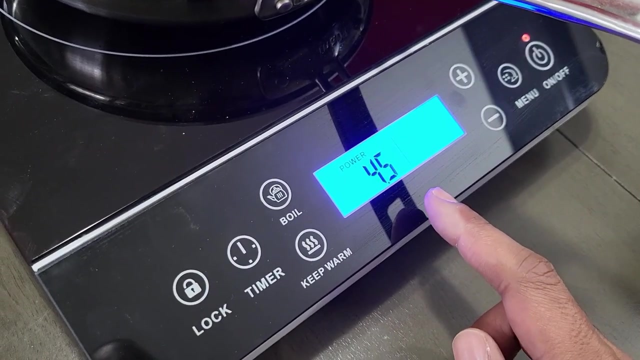 Five, nine, seventy four. Okay, I heard some weird double beep, but it still did it. Let's go up to 4.5 and see what it does. Okay, this is getting an error. I'll see if it does it again. They had error three. 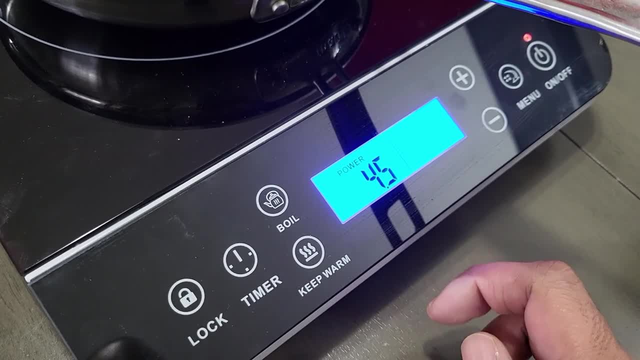 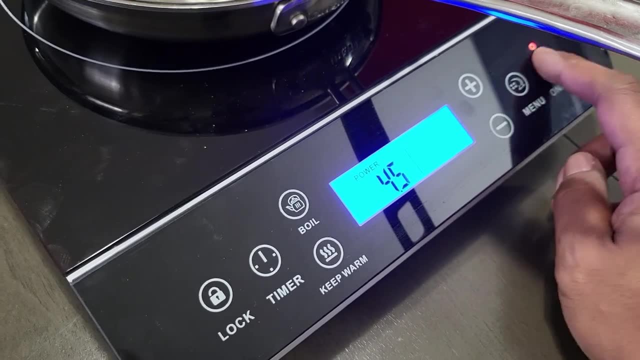 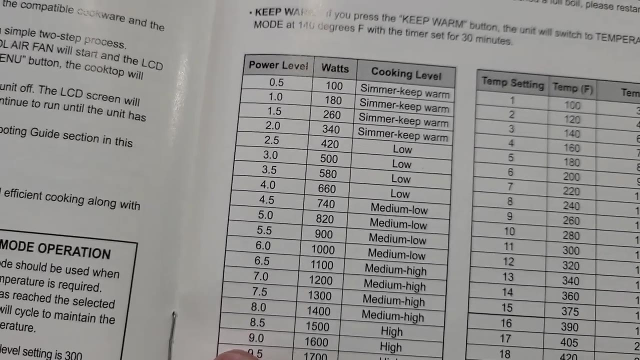 I may need to grab my instruction booklet and see what that means. Error three: Okay cool, So we're gonna turn it off. Let's see what that area is. We're trying to find some error codes here. Oh, look at that. It actually talks about what the power levels mean: simmer, keep warm a hundred watts.